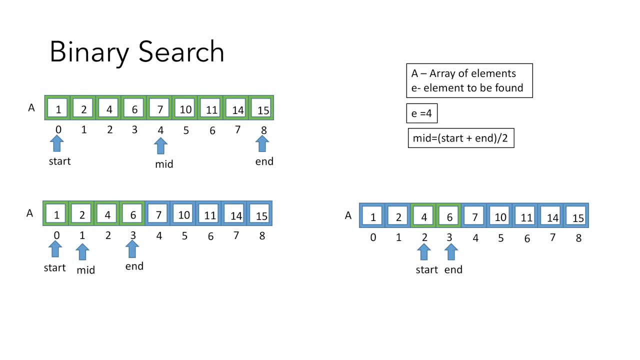 to mid plus 1, that is start, is now pointing to the index 2.. And again calculating mid, which would be 3 plus 2 divided by 2, that is 2.. We find the element we were looking for, That is, 4, at the middle index. So we can simply say that we found the element 4 at index 2.. 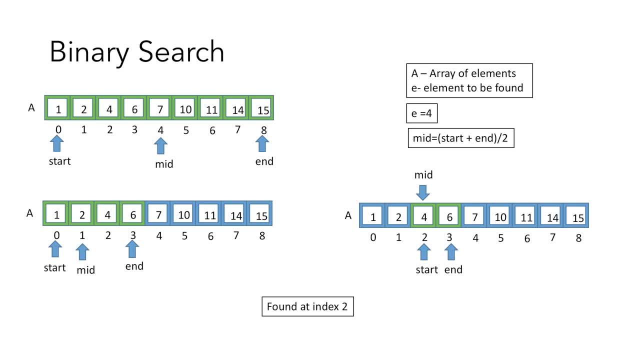 Now, if we look closely, to find the element 4, we divided the array into 2 parts at every step, and it took us 3 steps to find the element 4.. So now let's see how we can improve this using interpolation search. So the first requirement for interpolation search is that the elements 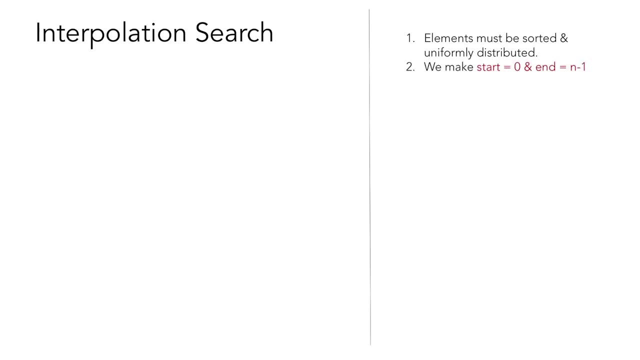 must be sorted and uniformly distributed. Then we make a start variable equal to 0 and end variable equal to n minus 1, where n is the number of elements in the array. Now, instead of calculating the middle index in interpolation search, we calculate the position. 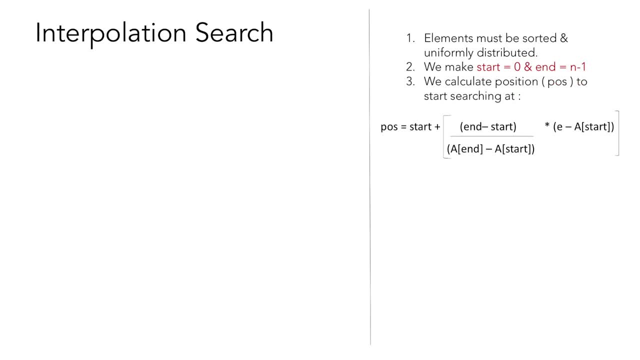 to start searching at using the formula position equal to start plus n, minus start divided by the element at end minus the element at start, multiplied by the element we are looking for, minus the element at start. index. In this formula, e represents the element at start. 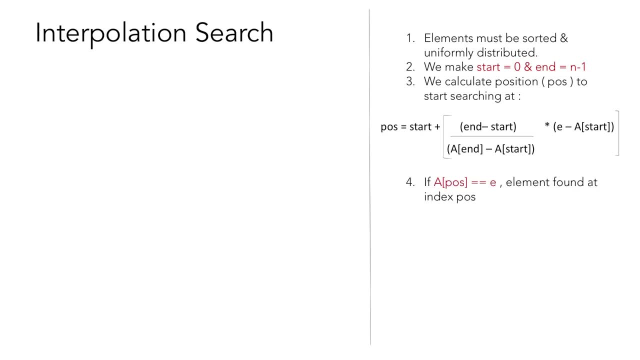 Now, after calculating the position, if the element at that position is equal to the element we are looking for, then we simply say that the element is found at index in the variable pos, which represents position. Otherwise, if the element we are looking for is greater, 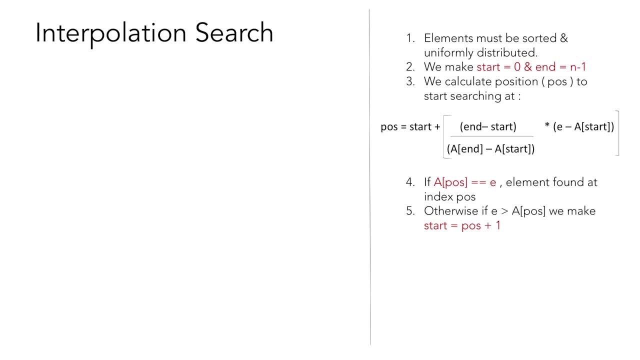 than the element at current position, we will make the start equal to current position plus 1.. Else, if the element we are looking for is less than the element at current position, we will make n equal to current position minus 1.. So let's try this out using the previous example, and again we are looking for the element. 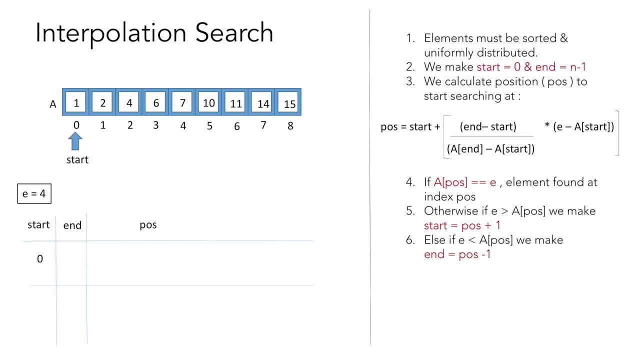 4 and initially start is equal to 0 and end is equal to n minus 1, that is 8 in our example. Now, using the formula, we will calculate the position to look for the element, and by putting the corresponding values of start, end and e in the formula, we get 0 plus 8 minus 0. 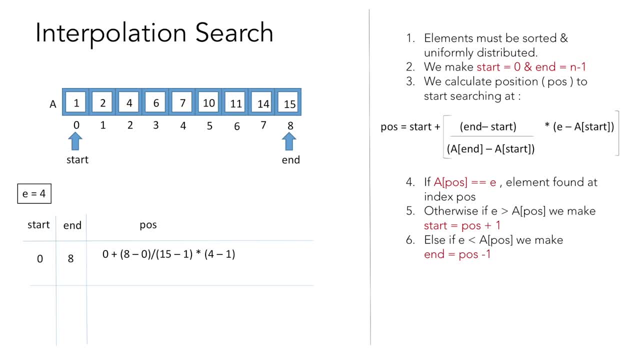 divided by 15 minus 1, multiplied by 4 minus 1.. Which, on further solving, would be 8 divided by 14 multiplied by 3.. Now one thing to note here is we will calculate the division part in decimals, Otherwise the answer may turn out to be 0. So the value of position would be 0.57 multiplied by 3. 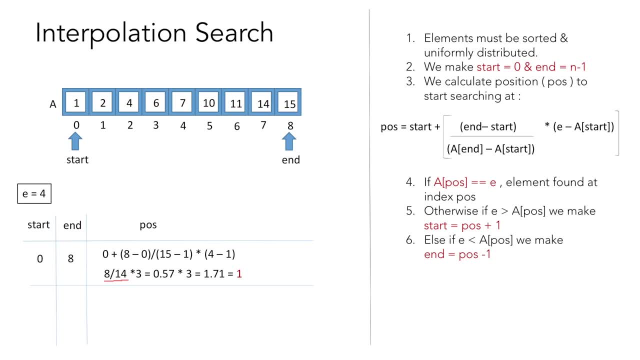 which is 1.71, and in the final answer we will take the integer value, which is 1.. Therefore, we now check the value at index 1, which is 2 and is not equal to 4, and as greater than 2, we will make start equal to current position plus 1.. 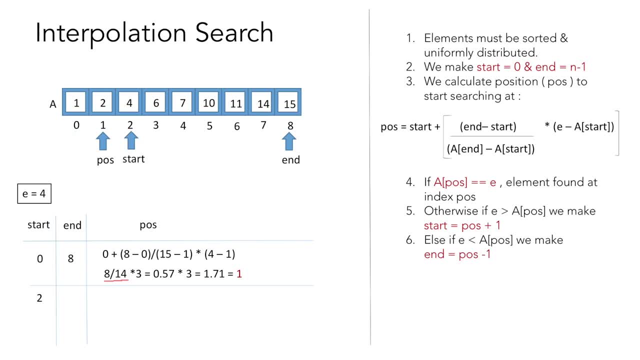 Therefore, start now has the index 2 and there would be no change in the value of end, which would again be 8.. And now we will again calculate the value of position using our formula and putting the corresponding value of start, end and e in the formula, we get 2 plus 8 minus 2. 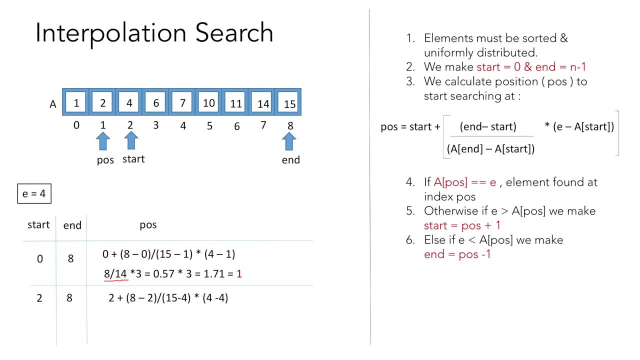 divided by 15 minus 4, multiplied by 4 minus 4, which would be 2 plus 6, by 11 multiplied by 0., Which is equal to 2.. So now we will check the value at index 2, and the value at index 2 is equal to 4, which. 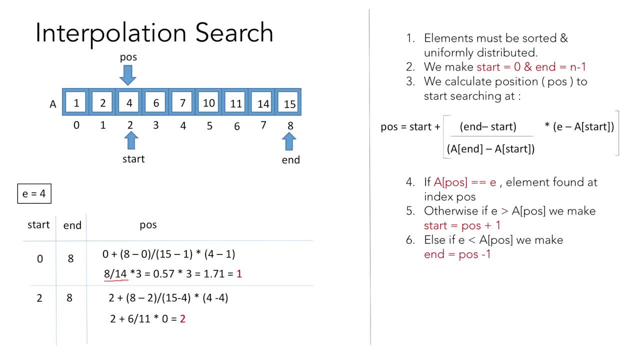 is the element we were looking for. So we can simply say that we found the element at index 2.. Now, if you remember, when we searched for the same element using binary search, it took us 3 steps to find the element 4, while with interpolation search we were able to find. 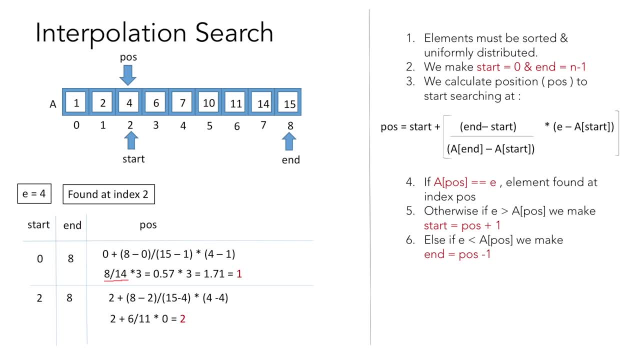 the element 4 in 2 steps. This is because with binary search we were always looking at the middle index, While with interpolation search we started looking at the index, which were closer to the element we were looking for. Now one last thing: If the element is not present in the array, we will perform interpolation search until 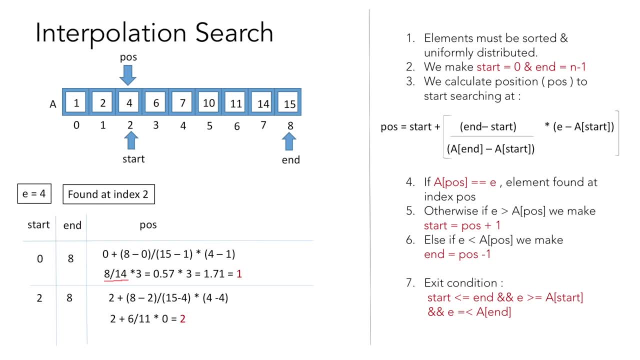 start is less than or equal to end, and the element we are looking for is greater than or equal to the element at the start index, and the element is less than or equal to the element at end. So now let's implement this using C++. We start by hide the element at start.